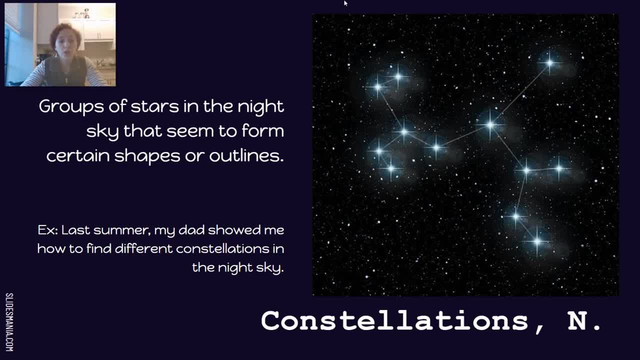 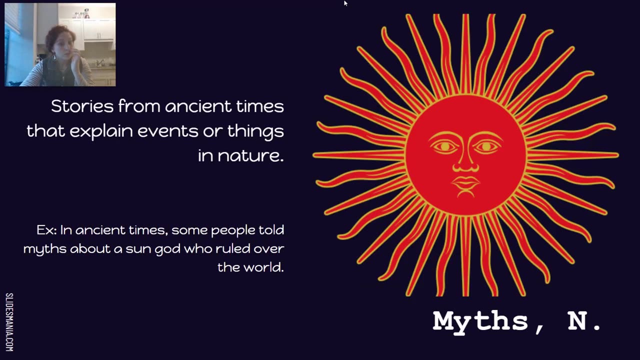 Constellations, Also a noun. Constellations are groups of stars in the night sky that seem to form certain shapes or outlines. Last summer my dad showed me how to find different constellations in the night sky. Myths- Another noun. Myths are stories from ancient times that explain events or 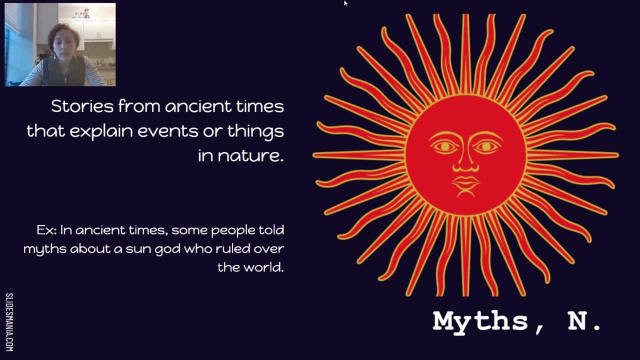 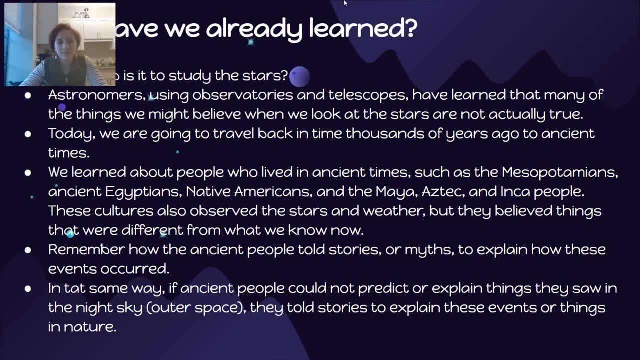 things in nature. In ancient times, some people told myths about a sun god who ruled over the world. So whose job is it? to study the stars? Astronomers, right, And astronomers using observatories and telescopes have learned that many of the things we might believe when we look. 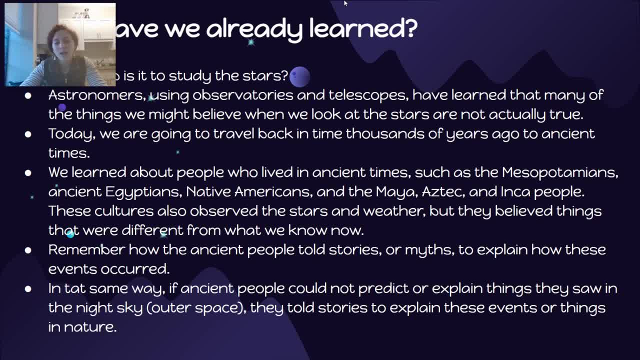 at the stars are not actually true. Today we are going to travel back in time thousands of years ago, to ancient times. We learned about people who lived in ancient times, such as the Mesopotamians, ancient Egyptians, Native Americans, the Maya, the Aztec, the Inca people. These cultures also. 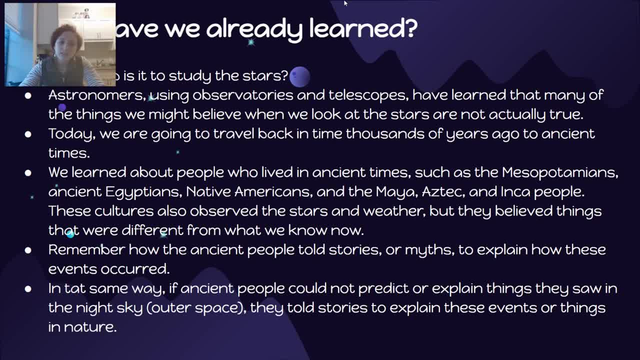 observed stars and weather, but they believed things that were different from what we know now. Remember how the ancient people told stories or myths to explain how these events occurred. Well, in that same way, if ancient people told stories or myths to explain how these events 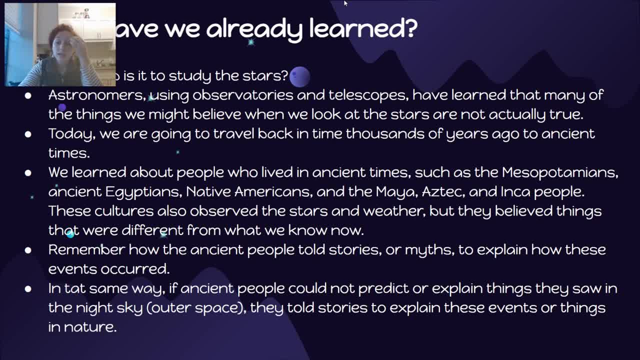 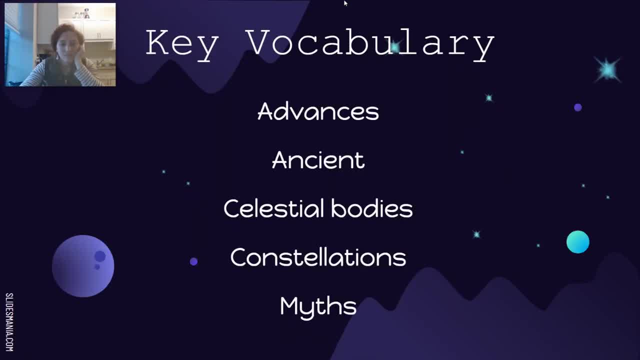 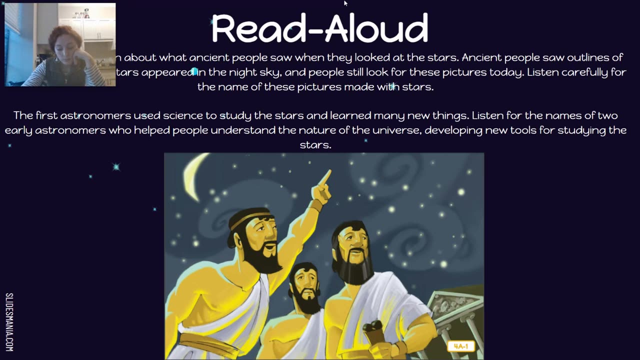 could not predict or explain things that they saw in the night sky. they told stories to explain events or things in nature. all right, remember our key vocabulary advances: ancient celestial bodies, constellations and myths. so we are now going to learn about what ancient people saw when they looked at. 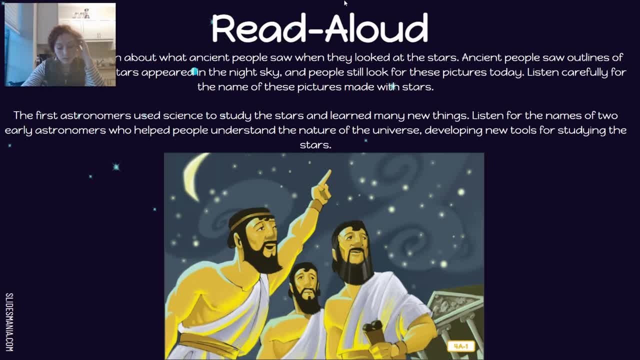 the stars. the ancient people saw outlines of pictures in the way the stars appeared in the night sky and people still look for those pictures today. I want you to listen carefully for the names of these pictures that are made with stars. the first astronomers use science to study the stars and learn. 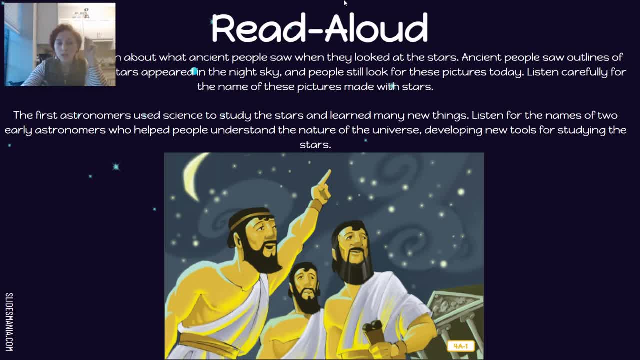 many new things. listen for the names of two early astronomers who helped people understand the nature of the universe, developing new tools for studying the stars. thousands of years ago people had no telescopes and no rocket ships. although people back then did not have the tools or knowledge that we have today, they 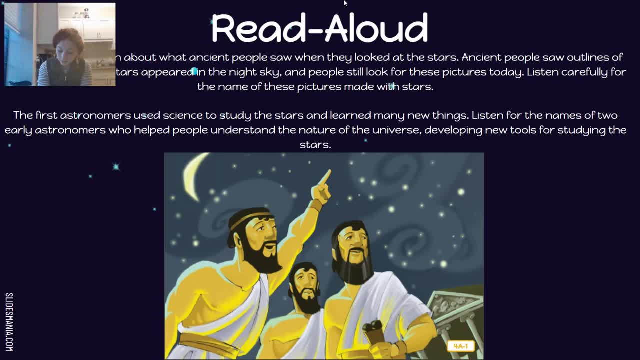 were just as curious about the stars and other celestial bodies, meaning objects found in space: the ancient Greeks, Arabs, Romans, Chinese, Egyptians, Turks, Mayans, Babylonians and countless others who lived long, long ago all the stars and tried to figure out what they were and why they were there. 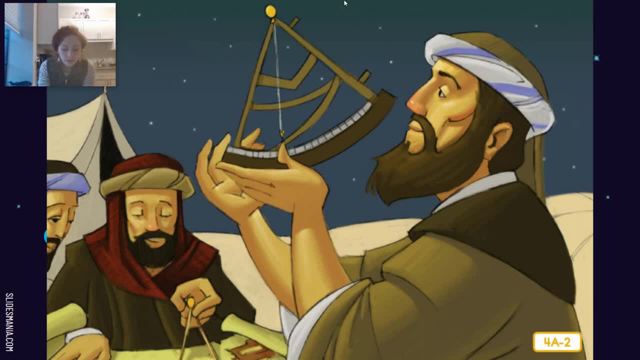 Although they did not know what the stars were made of or how far away they really were, the ancient people named the stars and mapped them out. We still use those names today. They figured out which stars appeared in the sky during certain times of the year, and even though thousands of 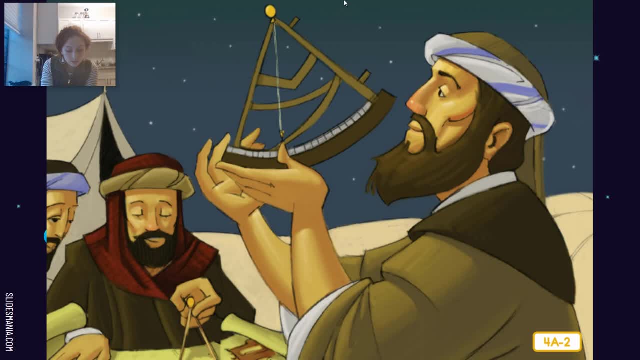 years have passed, on earth, the stars have basically remained the same. In other words, when you look up at the stars at night, you are seeing nearly the very same stars that the ancient Greeks, Arabs and countless others saw as well. So outer space has changed very little in all of those years. 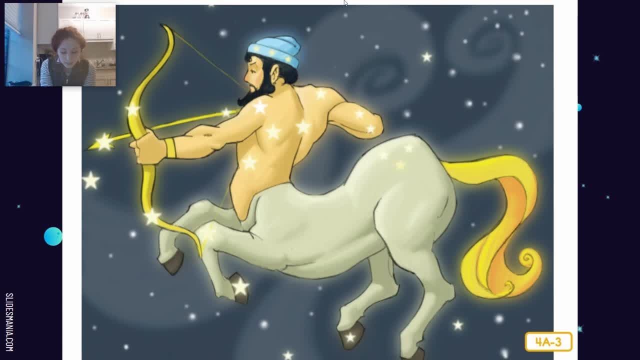 The ancient Greeks believed that the stars had been placed in the sky by gods. in order to tell stories and teach lessons, The Greek identified certain groups of stars in the night sky that seemed to form specific shapes. These shapes are called constellations. That's the name for the 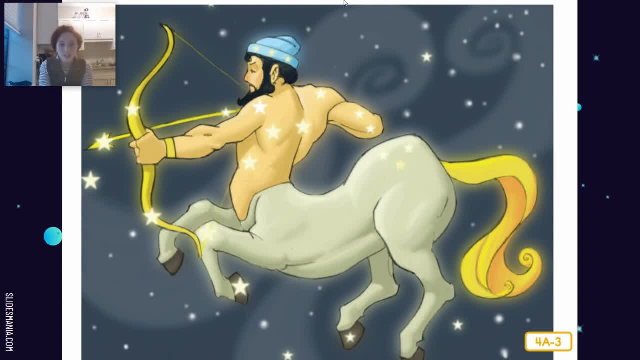 pictures that they saw in the stars. So constellations are the pictures that were seen in the stars. In the United States, Europe and many other parts of the world we still call the stars by the names that the ancient Greeks or Arabs. 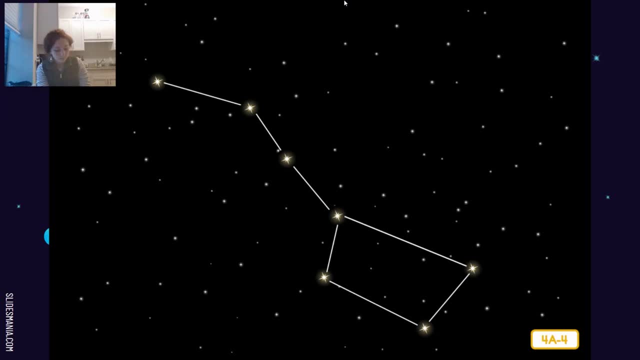 used so long ago. The Big Dipper is not actually a constellation in itself, but a part of a bigger constellation called Big Bear. That is why it's referred to as a group of stars in this readaloud- One of the first groups of stars that young. 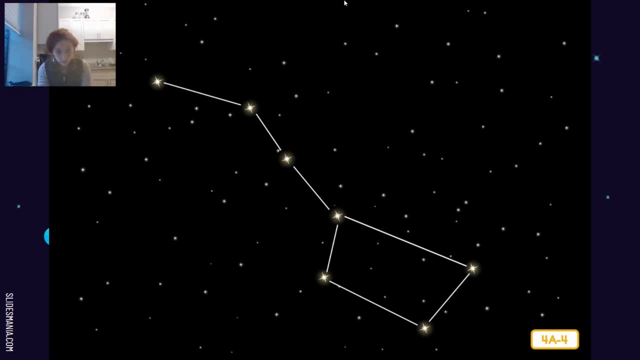 stargazers in the United States learn about is also the easiest one to spot. The Big Dipper looks kind of like a giant soup ladle in the sky. You might also think it looks like a pot, which is not true. What does it look like to you? The Big Dipper is made up of seven stars. 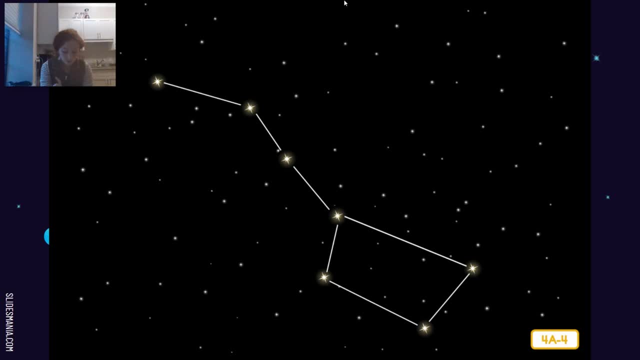 The Big Dipper looks different in the sky depending on the time of year. So if we were to flip that picture upside down, it might look like a hat. Okay, so I'll see if, maybe, if I can- oh no, there's no way for me to do that, But think about. 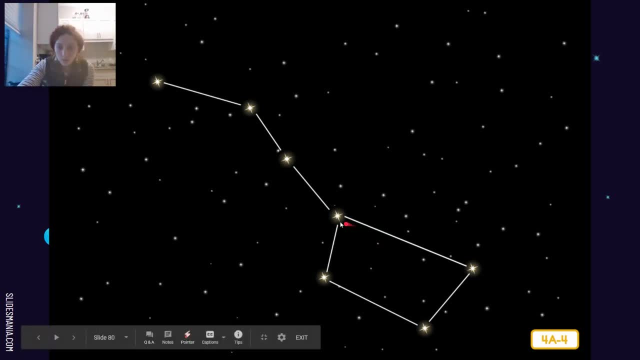 this. let me get my pointer. So this would be: if you flip it upside down, that would be the part that you put your head in, and then this would be the part that sticks out, right, Maybe? Okay, now let's see It said seven stars. so one, two, three, four, five, six, seven, Seven. 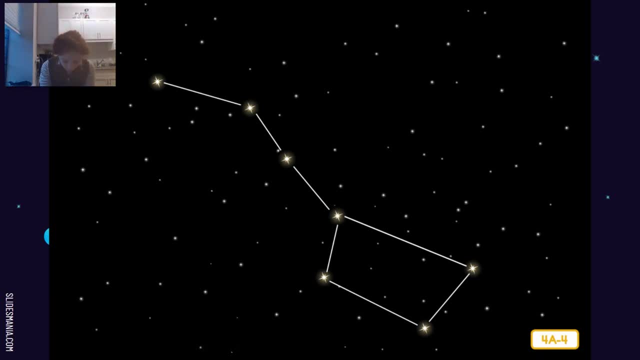 stars. Sometimes the Big Dipper looks right side up, sometimes it looks upside down and sometimes it appears to be standing on its handle. That is not because the Big Dipper moves, but because the earth is rotating on its axis and orbiting around the Sun. Remember we. 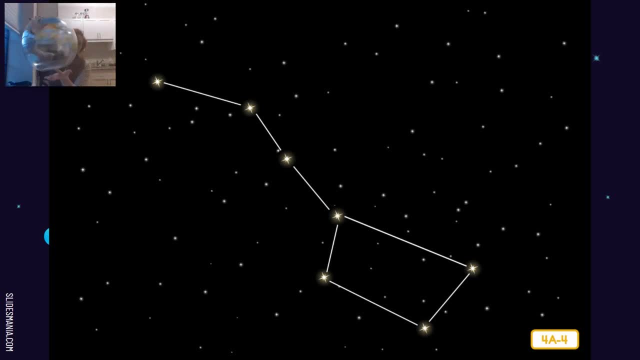 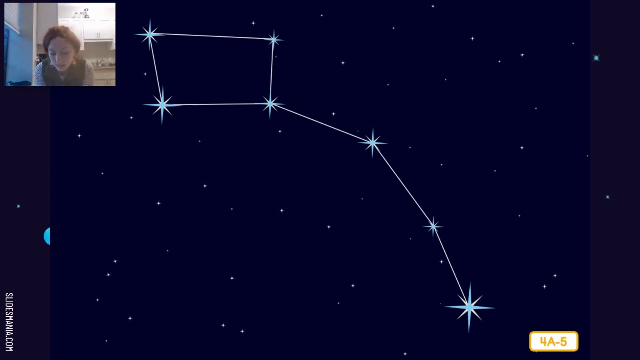 talked about rotating and revolving right, So the earth revolves and rotates at the same time. The Big Dipper Dipper has a friend called the Little Dipper. The Little Dipper also contains seven stars. The bright star at the end of the handle is special. It is called Polaris or the North Star. 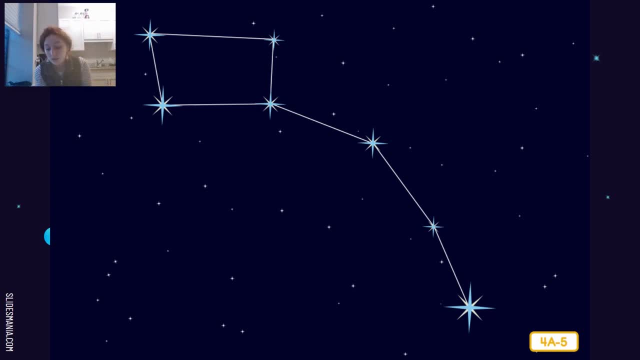 Basically sorry. unlike other celestial bodies, the North Star basically stays in the same place in the sky, as we observe it on Earth, always in the north. No matter where or how the Earth is spinning, that star always seems to be in the exact same spot, while the others seem to move. 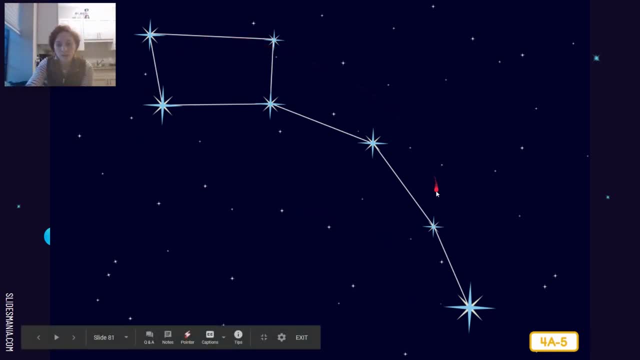 around? Which of these stars is Polaris? This one right here, the big, bright one at the end of the handle, Let's see It said seven stars: One, two, three, four, five, six and seven Exactly. 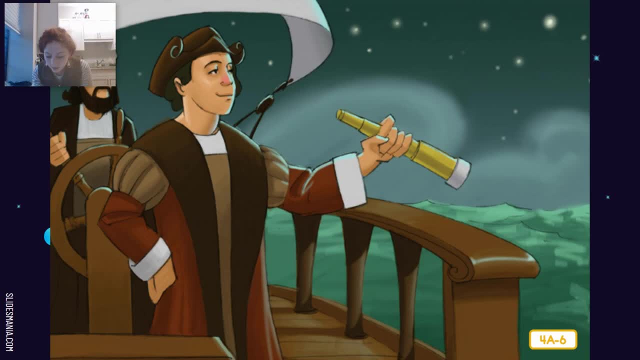 Since ancient times, people have relied on this star to find their way in the world. Knowing which way is north is the first step to figuring out which direction you are heading. Christopher Columbus and other sailors used to look at the North Star on starry nights out in. 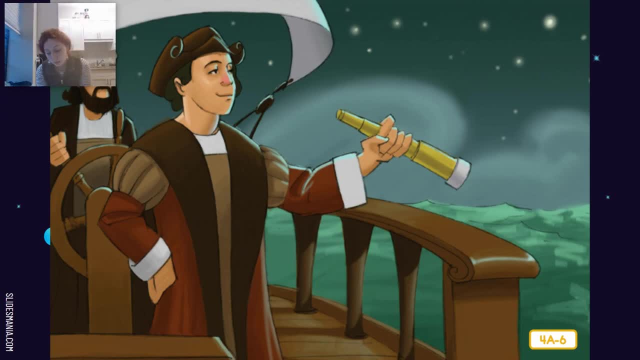 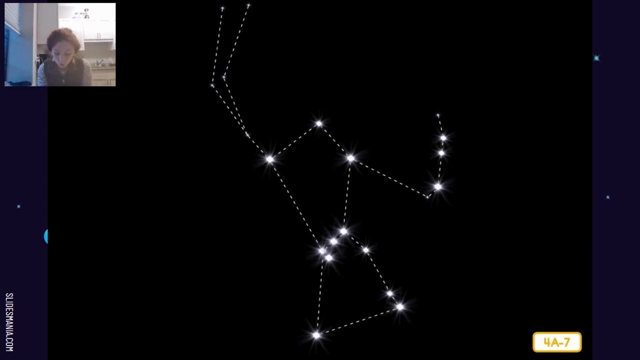 the wide ocean. Because Polaris is always in the north sky, Columbus would use it like a compass to navigate his ships north, south or east or west. This picture shows one of the most famous constellations of all: Orion. Orion is the story We're going to read. a little story. 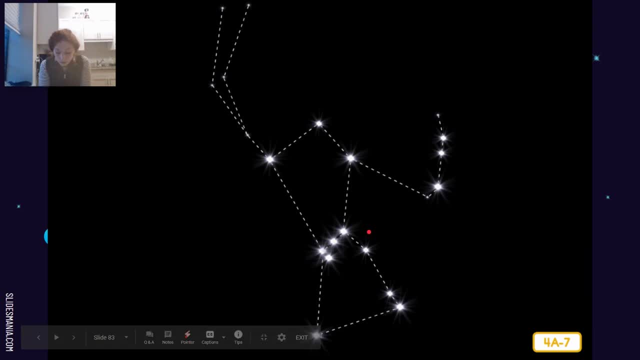 about it, but this is the one called Orion. Ancient Greeks told stories or myths about Orion, a famous hunter. Myths are stories from ancient times that explain events or things in nature. The constellation Orion is known all over the world. The constellation itself contains eight. 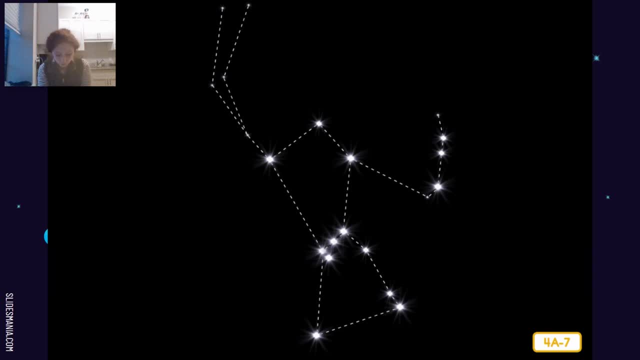 main stars. Orion's belt, made up of three stars in a row across his body, is the easiest to spot. As you can see, it takes a little imagination to look at these stars to see a hunter. This single star on the upper left is imagined to be the beginning of a raised arm which is holding. 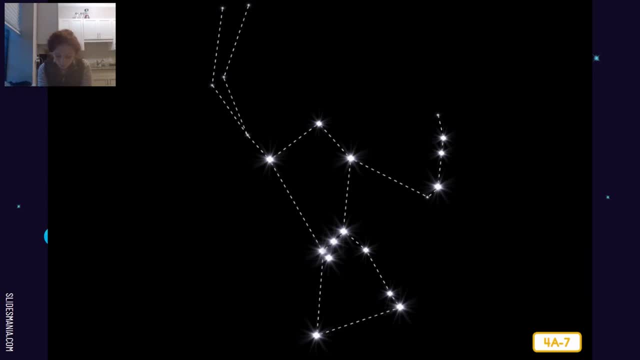 a club or a sword, With his other arm, imagined to be extended from a single star, holds a shield. So this is supposed to be like his body. right There's his belt. This is supposed to be his arm and he's supposed to be holding like a club or a sword. A club is kind of like a bat. This is his. 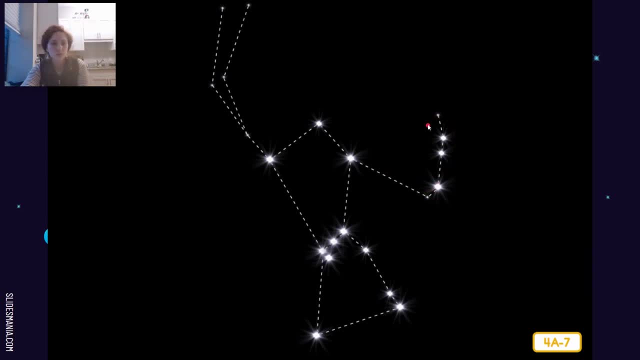 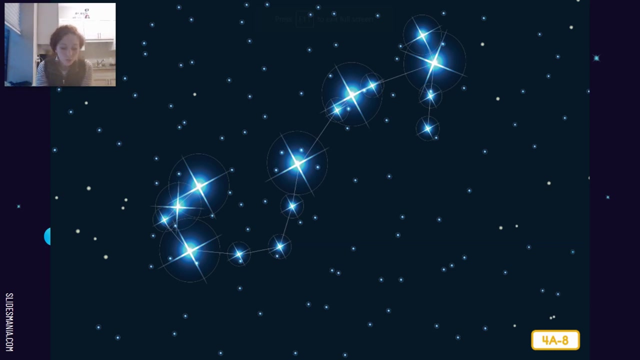 other arm and this is supposed to be his shield. okay, You kind of have to use your imagination, like it said. Okay, according to one myth, Orion bragged. he was such a good hunter that he could kill all the animals on earth. The gods decided to punish him by creating Scorpio, a giant scorpion that Orion. 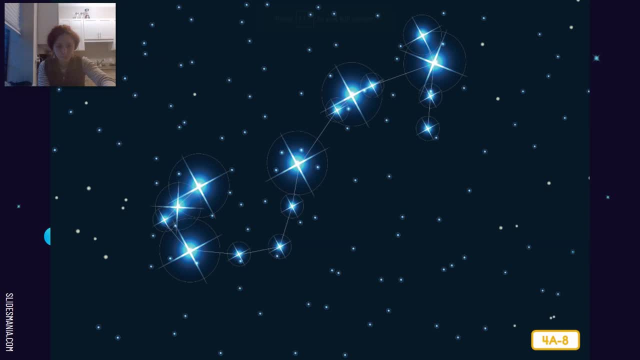 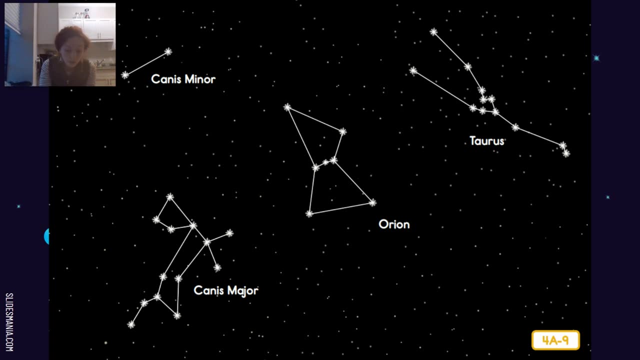 could not defeat. Not far from the Orion constellation is Taurus, which shows the head and horns of a mighty bull. It is often said that the hunter, Orion, is fighting the bull Taurus. So, according to the myths, Orion has a tough time up there. He's being chased by a giant. 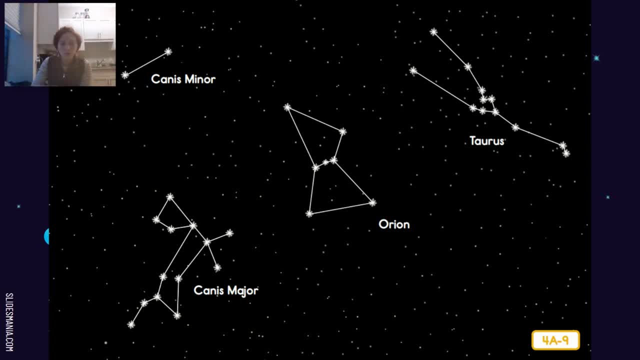 scorpion at the same time that he is fighting a giant bull. So this is supposed to be. this is Taurus, so that's supposed to be the bull. okay, Those are his horns, and then there's Orion, okay. 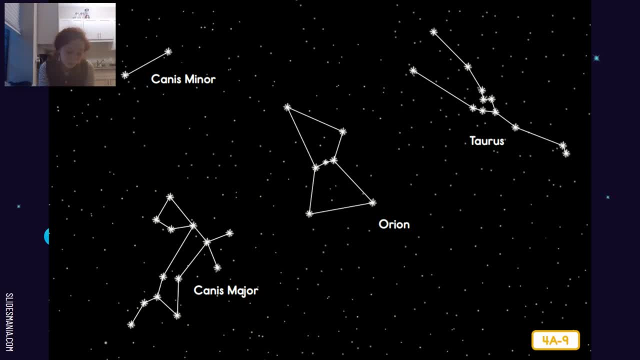 So on this day, Orion has a couple of friends, his two loyal hunting dogs, Canis Major and Canis Minor. These are Latin words: Canis means dog, Major means big and Minor means small. So if Canis means dog, 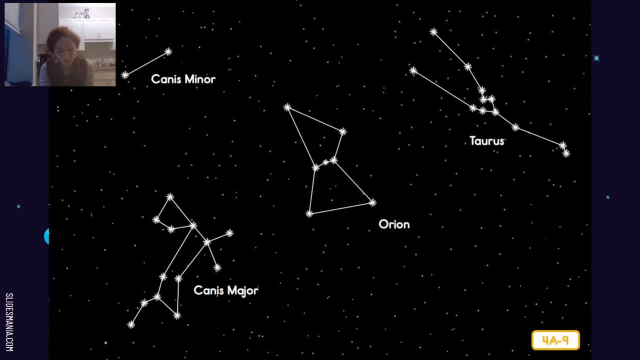 and Major means big, what does Canis Major mean? Big dog? And if Canis means dog and Minor means small, what does Canis Minor mean? That's a tongue twister. does Canis Minor mean Small dog? So here is Orion, Here's the bull. This is Canis Minor. So 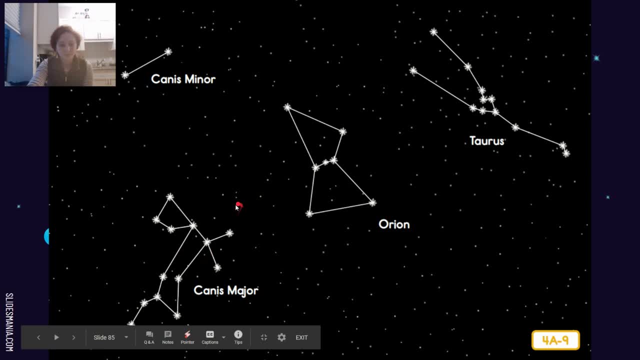 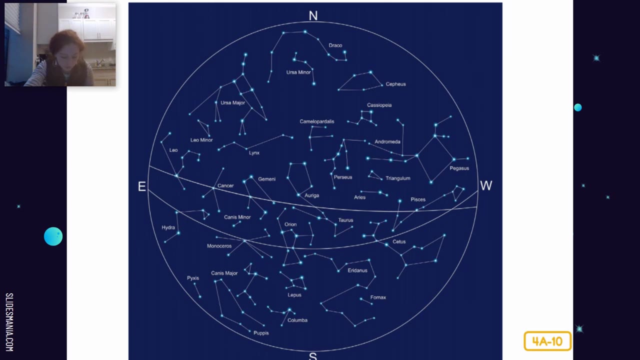 this is little dog and this is Canis Major big dog. Okay, These dogs follow Orion through the sky helping him to fight Taurus the bull. There are 88 major constellations and most people around the world use the same basic list When these constellations were first named most ancient. 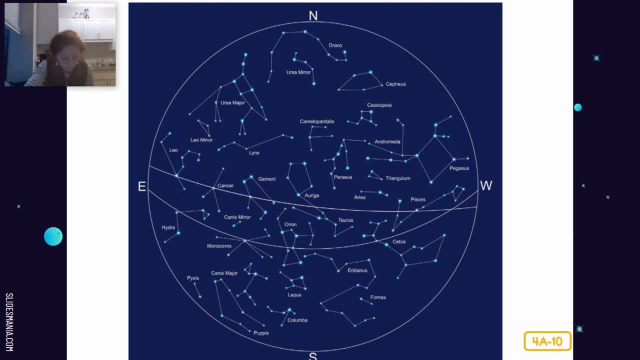 people could only guess what stars actually were. Ancient people told stories and myths based on what they could see with their own eyes when they looked up at the sky. But we have learned that there is so much more to space than meets the eye. In fact, sometimes when we look into outer space, 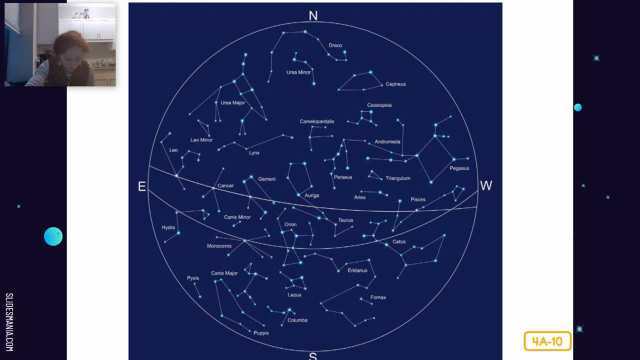 our eyes can play tricks on us. The first astronomers began using mathematics and science to provide different kinds of explanations than the myth that ancient people told to describe what they saw in the sky. Rather than make up stories, astronomers develop hypotheses or scientific explanations based on the facts. 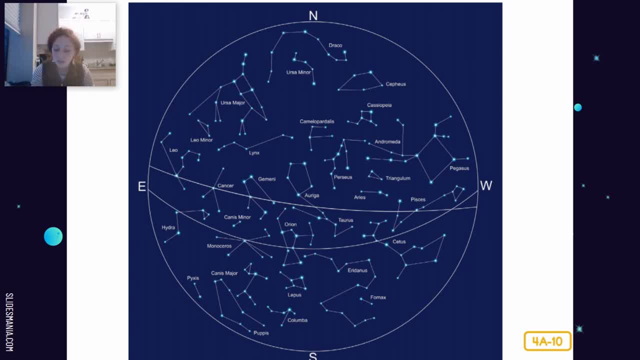 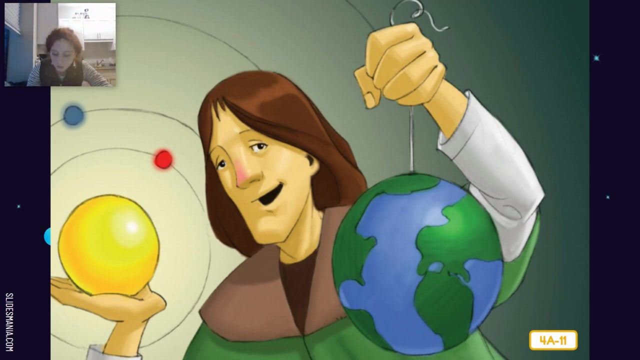 they discovered about outer space. So a hypothesis is different from a story because a hypothesis can be tested. Sorry, a hypothesis is one, Hypotheses is multiple hypothesis. Okay, Here we go. For example, ancient people saw that the sun rose on one side of the sky in the morning. 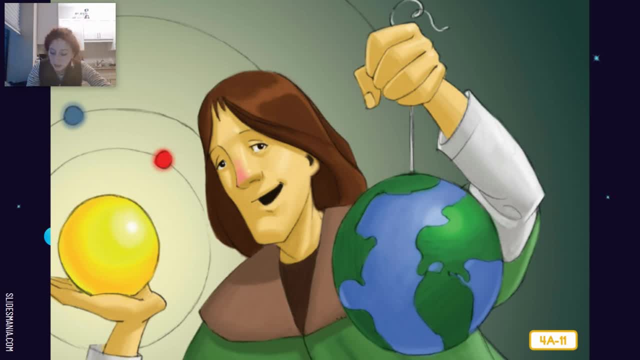 and set on the other side in the evening. Seeing the sun's movement across the sky caused ancient people to believe that the sun moved while the earth stood still. Ancient Greeks and Arabs, and, in fact, most people in the world, believe that everything in the universe, including the sun, 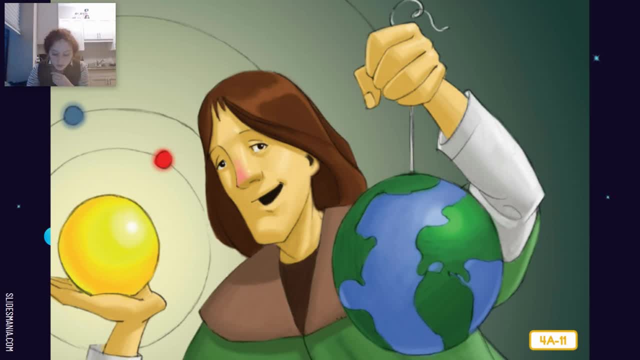 and all the stars revolved around the earth. It took thousands of years before anyone believed that the opposite was true. So, for example, ancient people saw that the sun rose on one side of the sky and it was true that the earth in fact revolved around the sun. 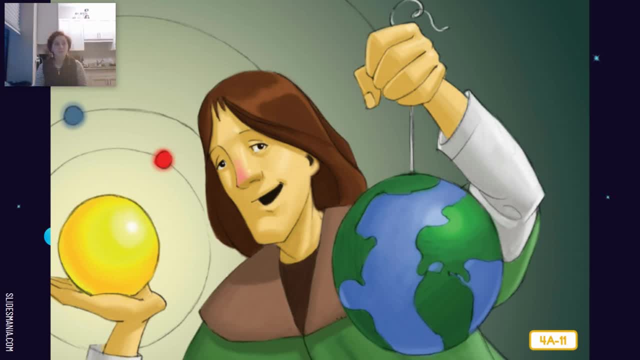 So remember, we know now because of science that the earth is the one that's moving right And that the sun stays still. But way back then, because of what we see in the sky from here on earth, it looks like. 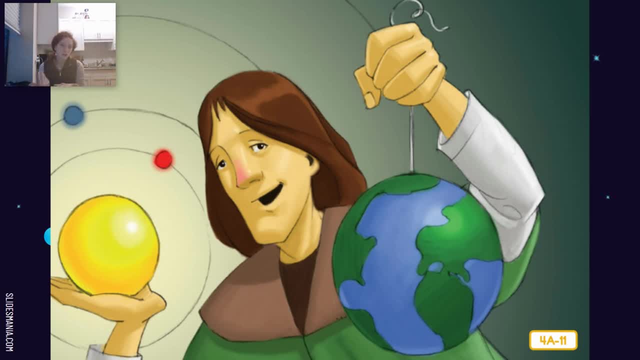 the sun is moving and the stars are moving right, But we know now that that's not true. This discovery was made by an early astronomer named Niklaus Copernicus. Can you say that, Niklaus Copernicus? Copernicus was the first to use science. 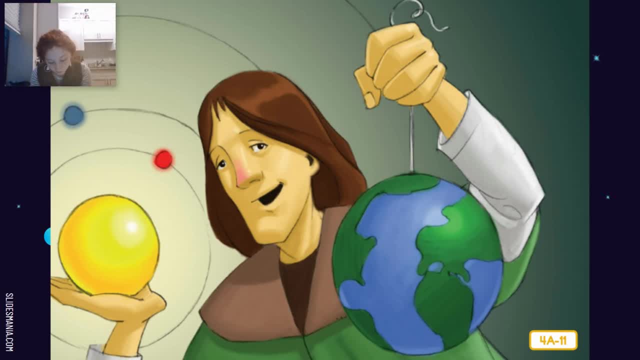 to explain that Earth actually revolves around the Sun. Unfortunately, hardly no one believed him at the time. That was about 500 years ago. So 500 years ago they didn't really believe him. They're kind of like: yeah, okay, bud, Another. 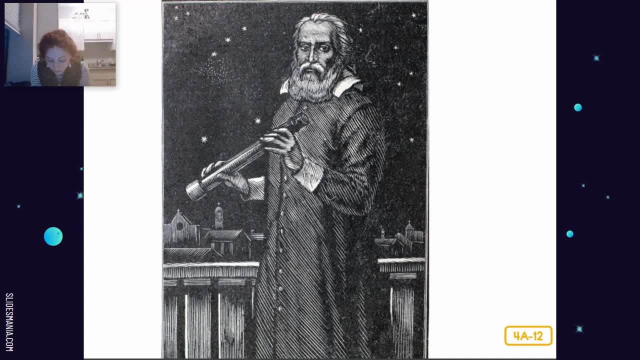 astronomer named Galileo came after Copernicus and he believed what Copernicus said about the Earth revolving around the Sun. He invented telescopes that helped astronomers prove that Copernicus's theory was true. What's a telescope? again, It's a tool to help us see the stuff that's in space. 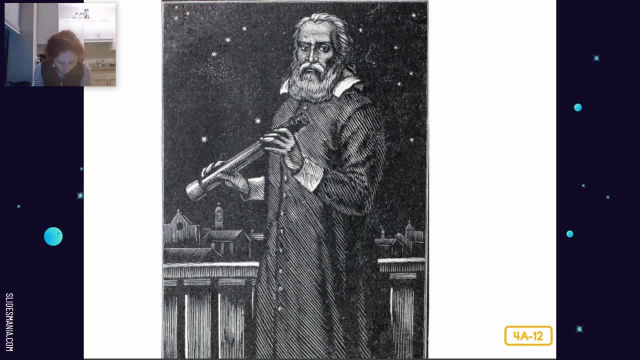 right, It magnifies it or makes it look bigger. Although Galileo did not invent the first telescope, he did invent very powerful telescopes that helped him and other astronomers discover the Earth. But he also invented the first telescope to help astronomers make many important 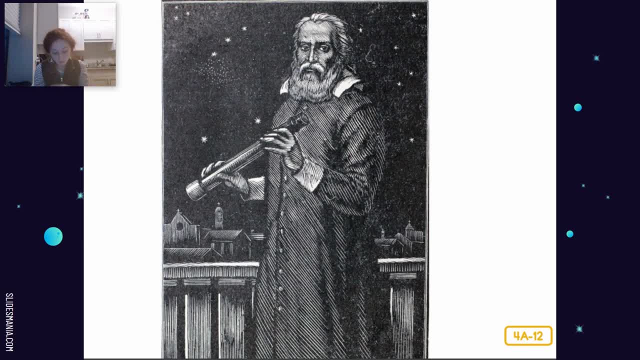 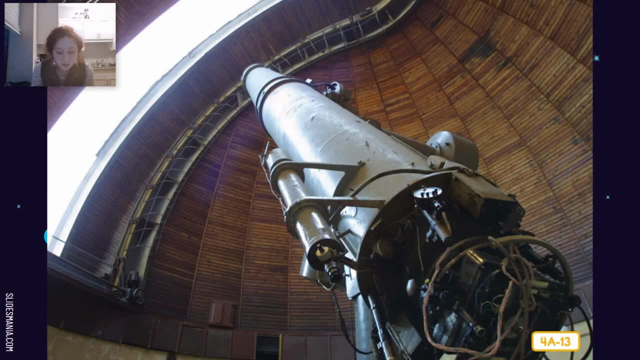 discoveries about space. For this reason, he is considered by many to be the father of modern astronomy. Since the time of these early astronomers, people have gained an incredible amount of knowledge about the stars and universe, and now use tools like telescopes to expand the knowledge each day. Copernicus. 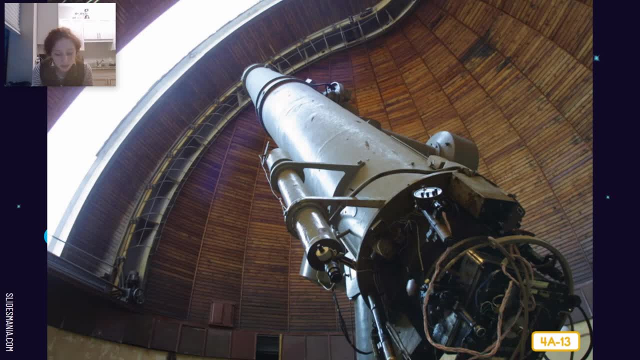 and Galileo would be amazed by the advances or progress people have made in astronomy over the past century, which means 100 years. Compare this incredibly large modern telescope to the one that Galileo was holding in the last picture. So this is the one that we have now, and that's the kind of one that they used to. 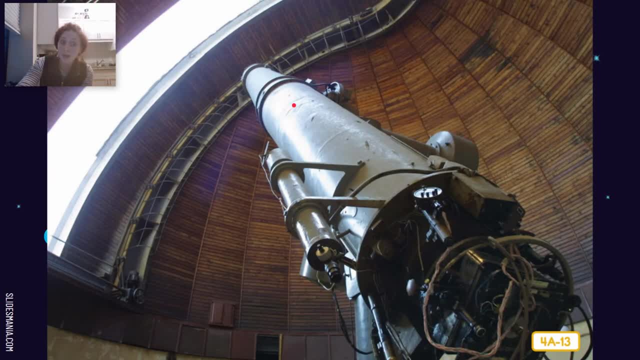 have. so ours is way bigger and way more complex, so we probably get better pictures with this one. Astronomers today use telescopes like this one to study the stars and other distant parts of outer space that Galileo may have never had. 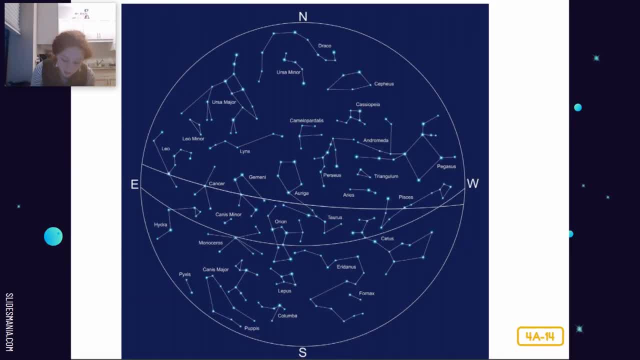 imagined. Yet even as we have gained new knowledge of outer space, our understanding of the stars is still built upon the stories and knowledge passed on by other people for thousands of years. Next time you find a constellation in the sky, you will know that other stargazers have been studying and 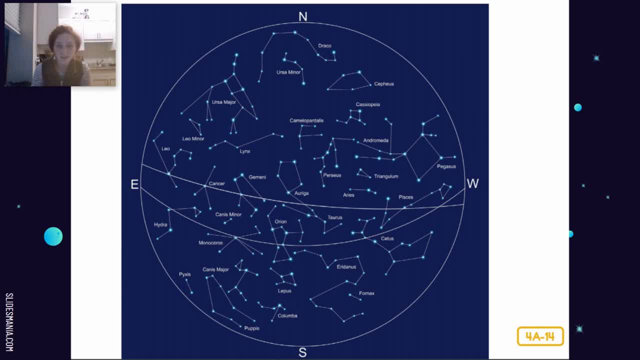 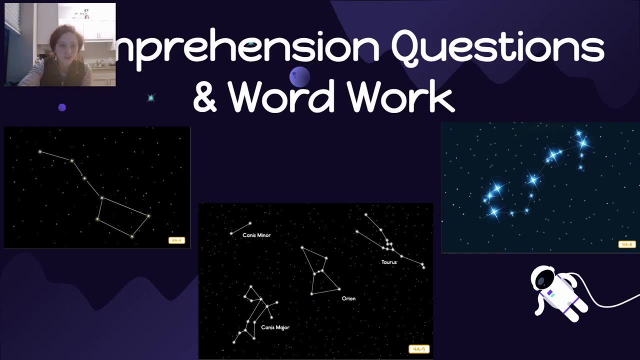 telling stories about that same group of stars for thousands and thousands of years. Isn't that pretty cool that people who lived thousands and thousands and thousands of years ago saw the same thing in the sky that we do. I think that's awesome. Okay, let's do some comprehension questions. 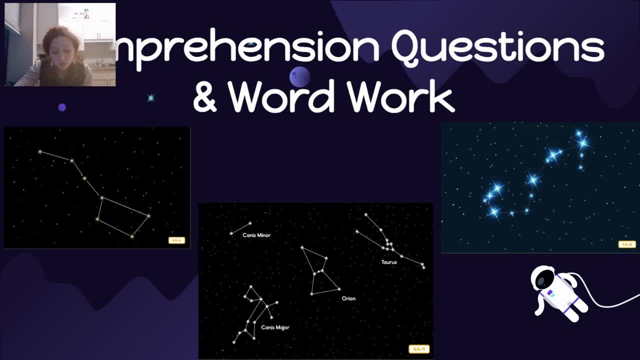 and our word work. So the ancient Greeks believed that gods put certain groups of stars together in the sky in order to make pictures that would tell stories and teach lessons. What are those pictures called? Starts with a, C: Constellations. Okay, So which constellation is this? That is the Big Dipper. Okay, What about? 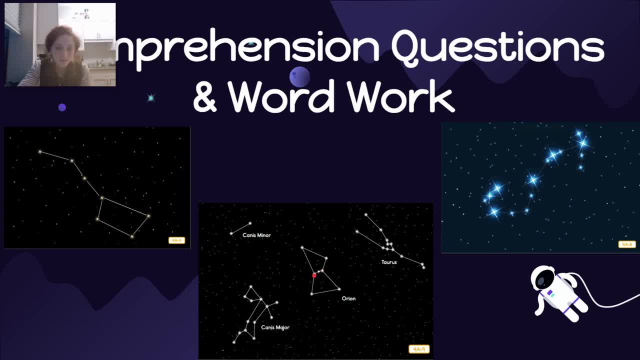 this one. Look at those three that make up a belt. This is Orion. And do you remember the name of the bull that was chasing him, Taurus? And then who are these? These were his friends, Canis minor and Canis major, Right. And then who's this? This is the one that's chasing Orion. 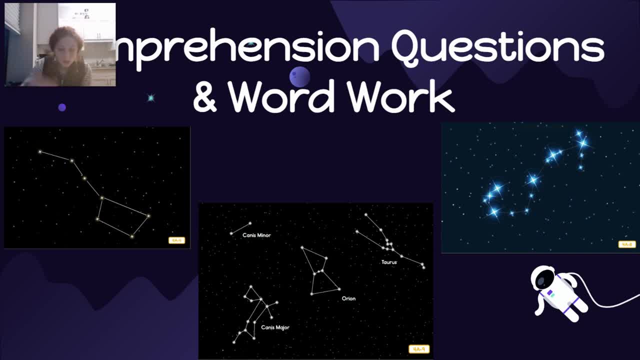 Scorpio, right. So now talking back about the Big Dipper. Why is this group of stars called the Big Dipper? Because it looks like a giant ladle or pot, right. And what's so special about Polaris, which is? 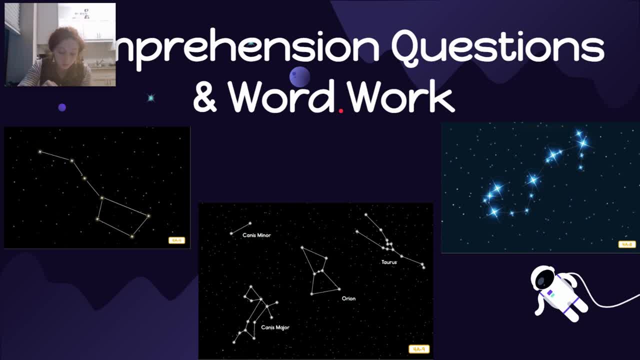 that star that is on the bottom of the handle of the Little Dipper Polaris. the North Star always stays north, making it a good star to use for navigation or directions. What astronomer was the first to say that the Earth revolved? 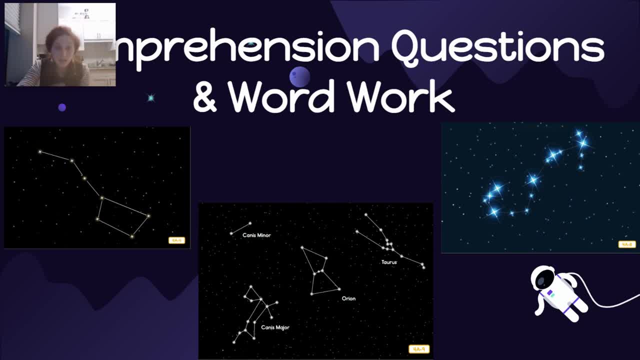 around the sun- Copernicus, but Galileo, Oh Galileo- helped prove that he was right. okay, We also learned about another important astronomer, Galileo. What invention did he improve upon that helped astronomers make new discoveries? Telescopes. In the Read Aloud, you heard the ancient. 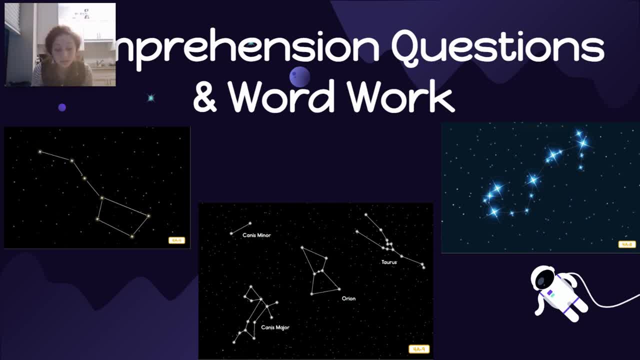 Greeks, Arabs, Romans, Chinese, Egyptians, Turks, Mayans, Babylonians and countless others all studied the stars. Say the word that is the word that starts that. Please say the word. that is the word that starts long. Please say the word that is the word that starts long. 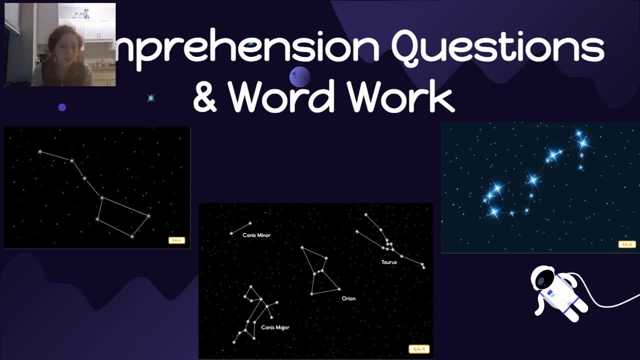 ancient with me? ancient. can you say it in a whisper voice? can you say it in a mouse voice? can you say it like you are ancient ancient. ancient is something very, very old, or from a very, very long time ago. okay, you may remember, we studied an ancient. we studied ancient Egypt and Mesopotamia to ancient. 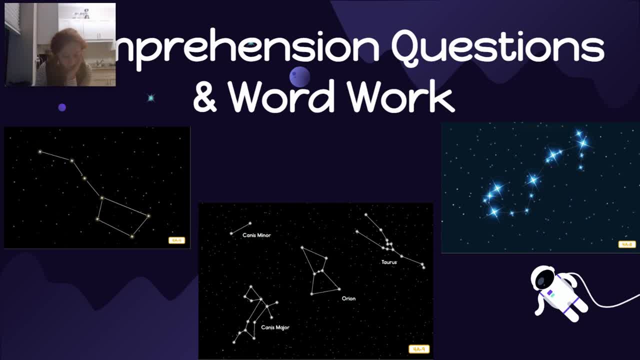 civilizations from thousands of years ago. so the opposite of ancient. so remember, ancient is really really old. the opposite of ancient is modern, which means new. okay, I'm gonna give you some sentences. okay, if it is something that is ancient, you're gonna say that is ancient. if it is something that is: 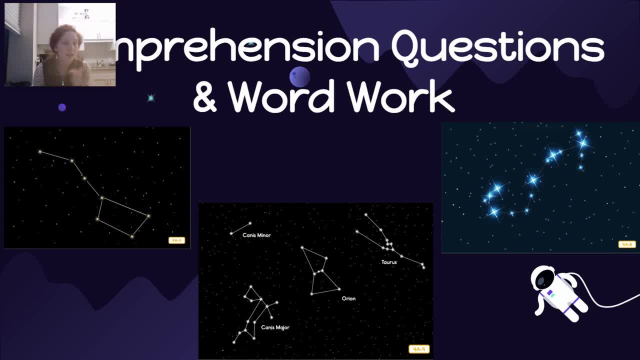 modern or new. you're gonna say that is modern. okay. when people want to talk about something, they want to talk about something. they want to talk about something to someone who lives far away. they call them on a phone or write an email. that is modern. okay, they did not used to have that. that's not super old, okay, barley? 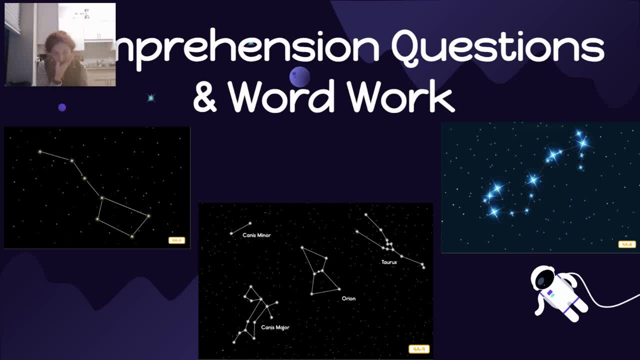 was used to trade in Mesopotamia. that is ancient. people keep food fresh in a refrigerator or a freezer. that's modern. people told stories about a hunter named Orion. to explain a set of stories about a hunter named Orion. to explain a set of stories about a hunter named Orion. to explain a set of stories about a hunter.